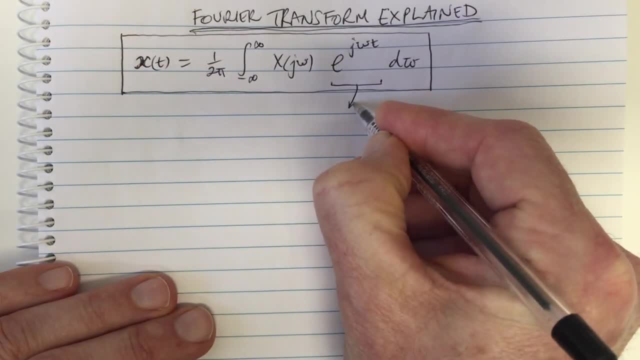 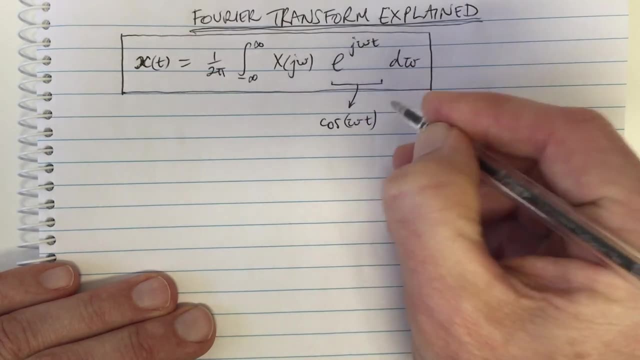 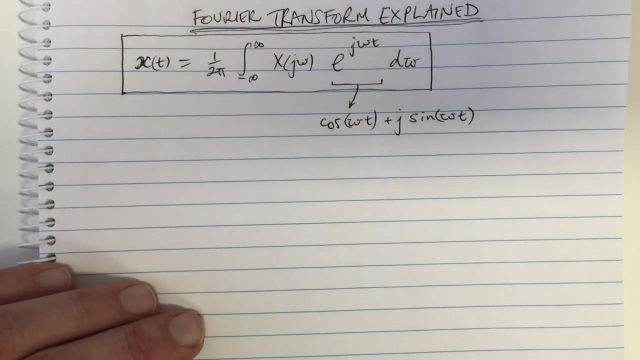 side depends on time and it's this function here. And what is this function? We remember this is cos of omega t, and that's the real function plus an imaginary of sine omega t. Okay, so this is a waveform And this is a waveform. One of them is the real part and the other is the 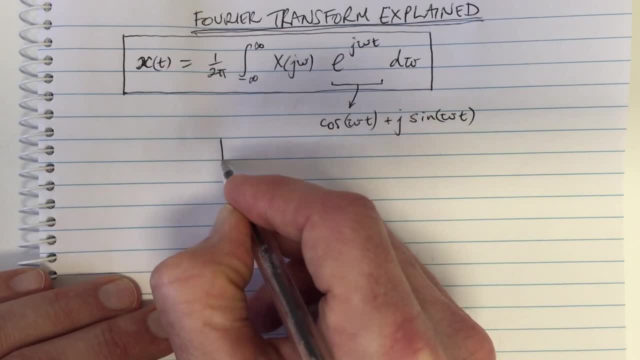 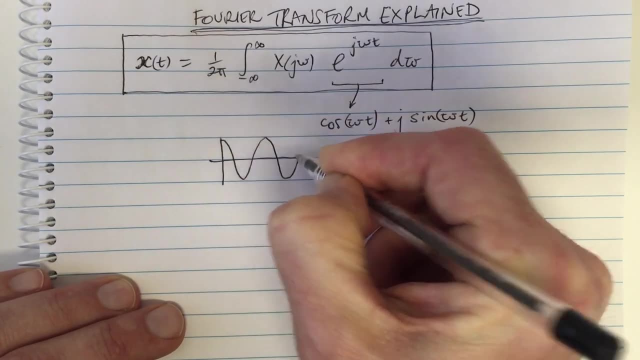 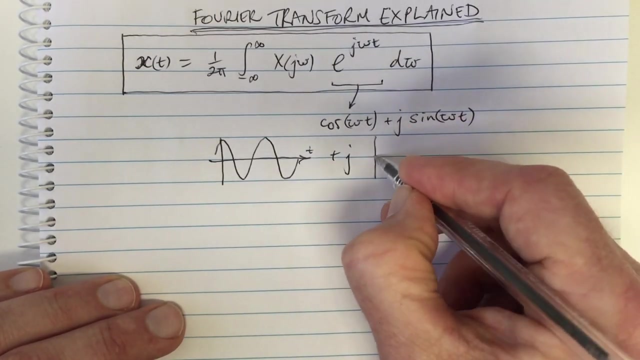 imaginary part And I always like to think of drawing out these waveforms. so let's draw the cos waveform here. This is a cos waveform, and plus a j, which is the sine waveform. This is a function of time And the sine waveform function of time, And they're at the same. 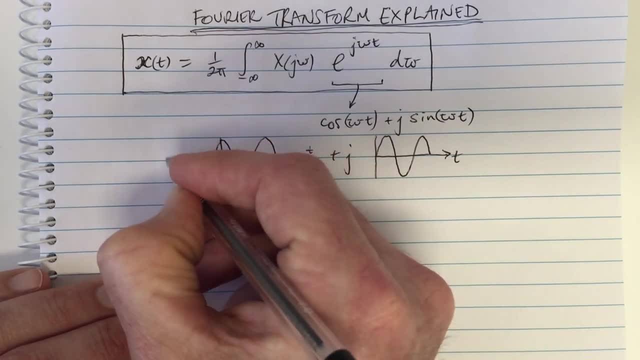 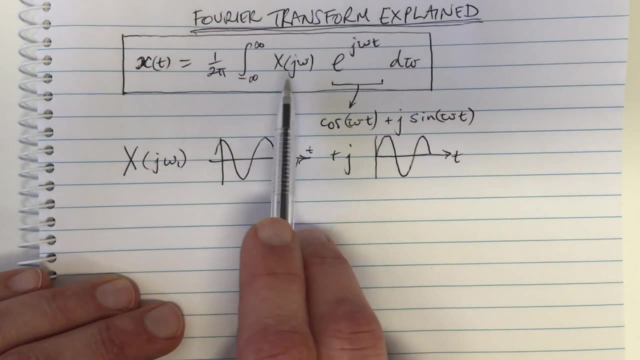 frequency, and I've drawn them there, And let's say that this is, This is omega 1, and so if we multiply by what this formula says is if we take one of these complex exponentials which has a real part, that looks like this: a function: 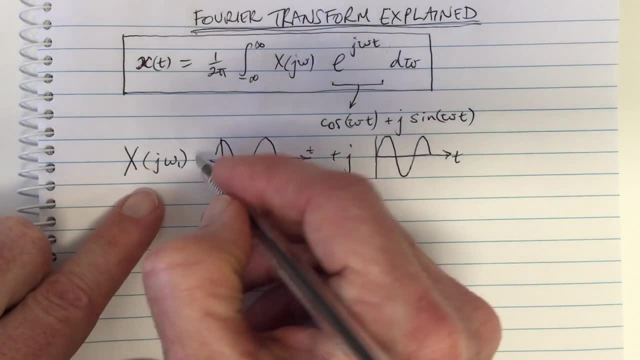 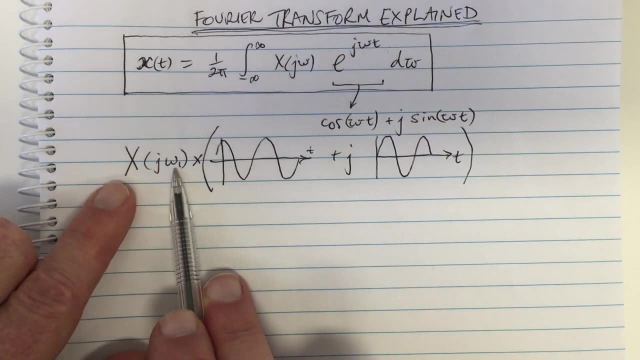 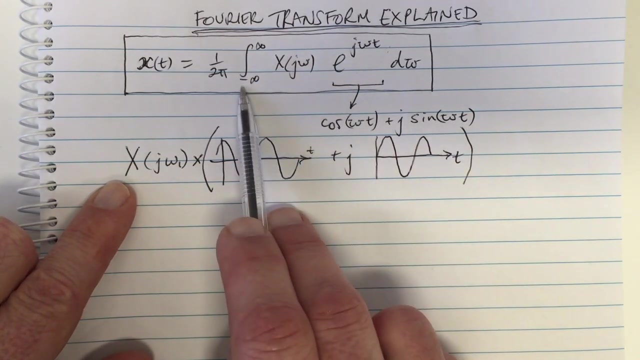 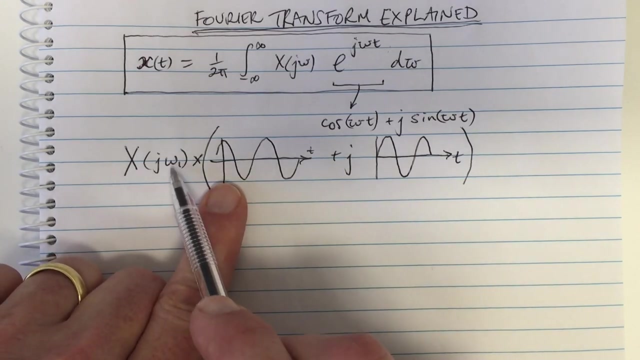 in time, an imaginary part like this, a function in time. if we multiply it by the value- this is a numerical value, a complex value at omega 1, then we will get one of the terms in this integral. So when I see this equation, I think about a cos waveform at a particular frequency. 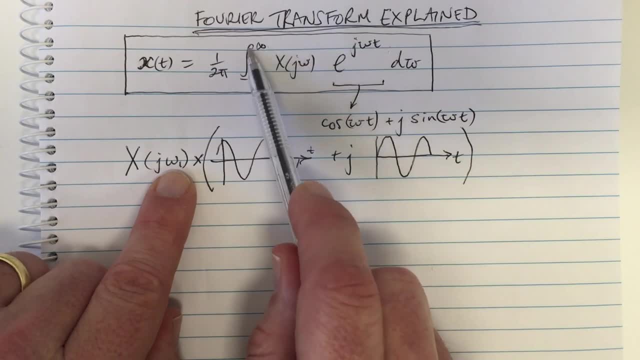 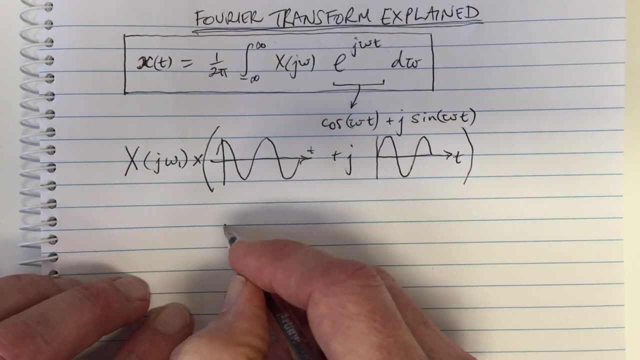 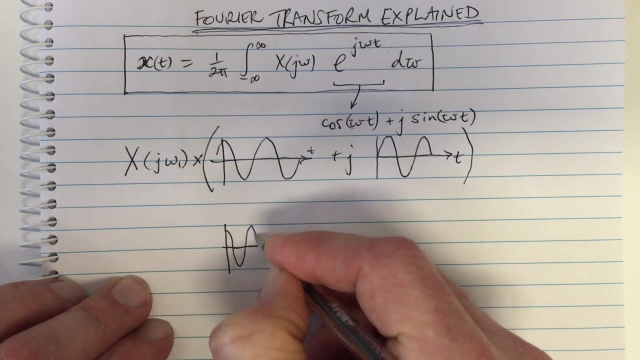 a sine waveform at that frequency and then we've got to have them all at different frequencies and add them all up. So let's draw one at another frequency here. So if we had a higher frequency, if frequency was increasing as we go down, then this is also a cos waveform at a higher frequency. 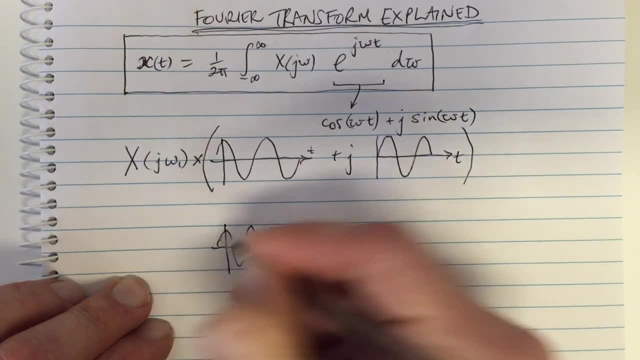 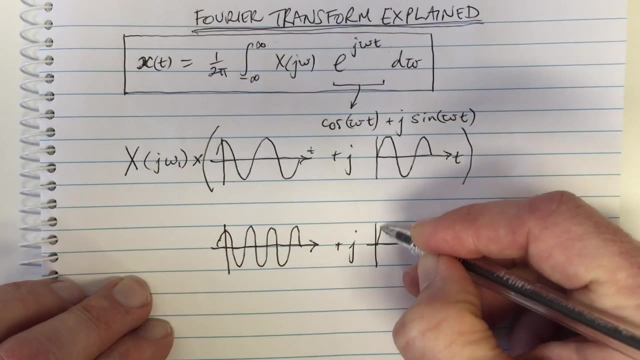 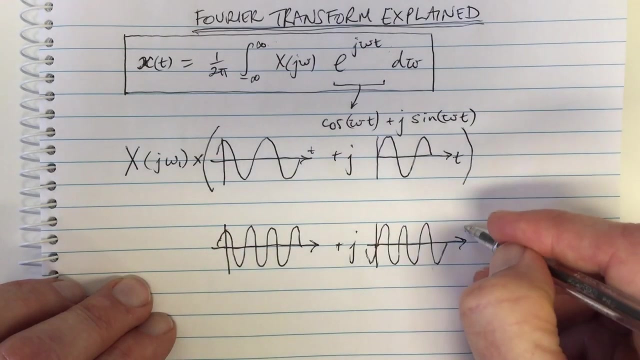 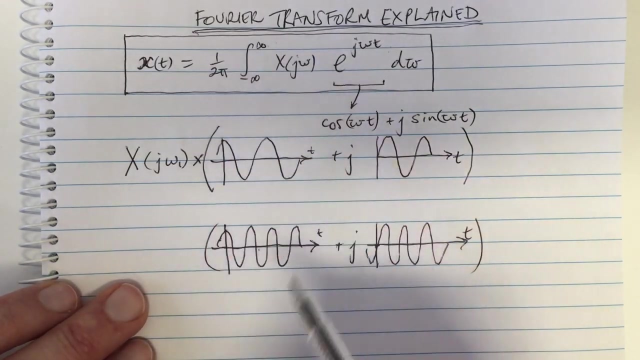 changes more quickly. So we have a sine waveform at a higher frequency plus j of the sine waveform at that same higher frequency. So the sine waveform crosses the zero time at zero, whereas the cos at the maximum. And again, those are two waveforms at another frequency in this summation. 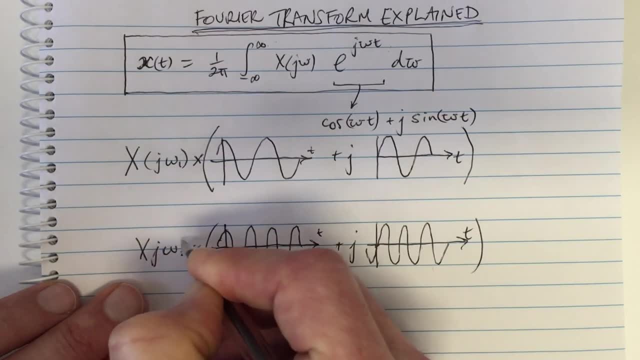 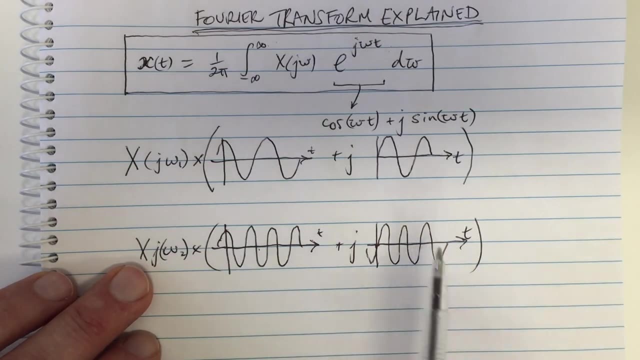 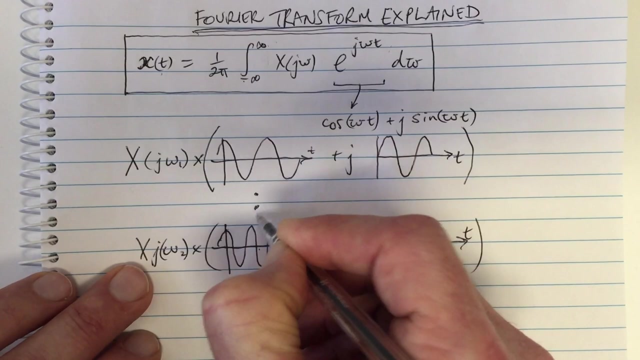 And again, if we multiply by the value, which is a weighting value, that weights the value that's the component of these waveforms in the signal that we are representing. OK, so we've got to add them all up. So these are. if we had all imagine all the ones in between there and, of course, beyond, 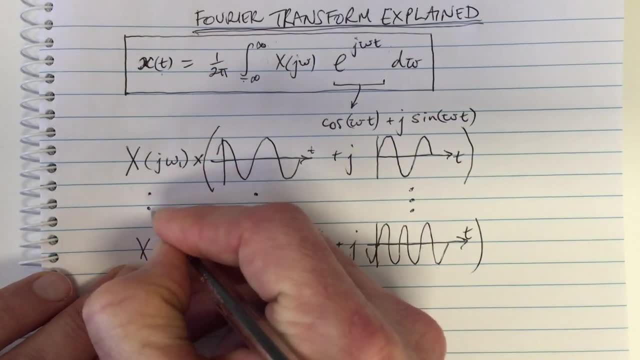 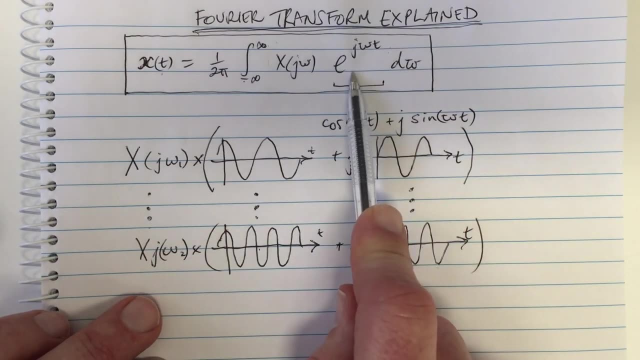 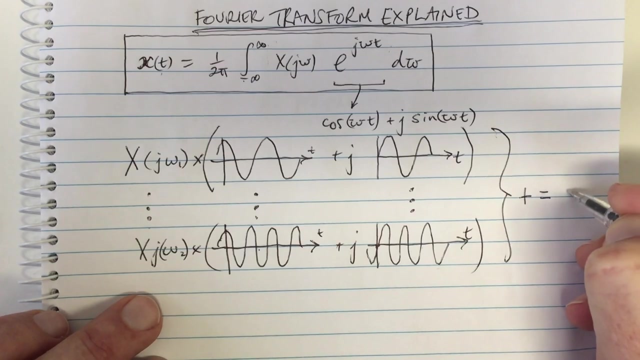 and so on, all the way from minus infinity to infinity, And what this equation says is these basis functions. so these complex exponentials are what we say are called basis functions. We add them all up, OK, And that gives us a time domain signal, which is the signal that we are representing. 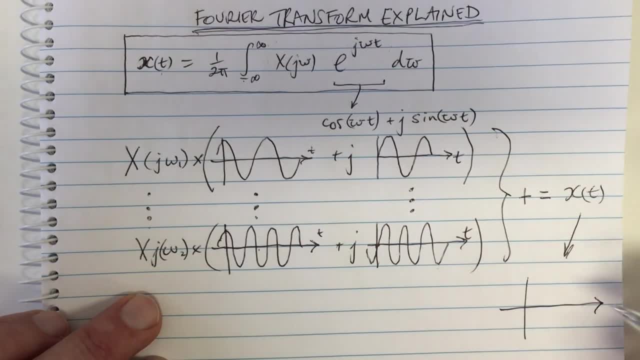 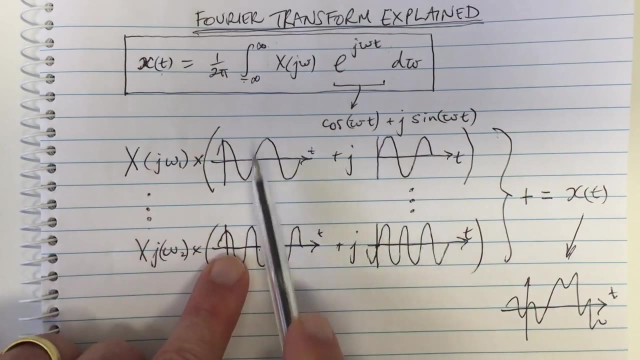 So this might be the recording of my voice speaking, or any time domain signal that has finite energy can be written as summations, this summation of these basis functions at all these different frequencies, all multiplied by a factor, And add it up. 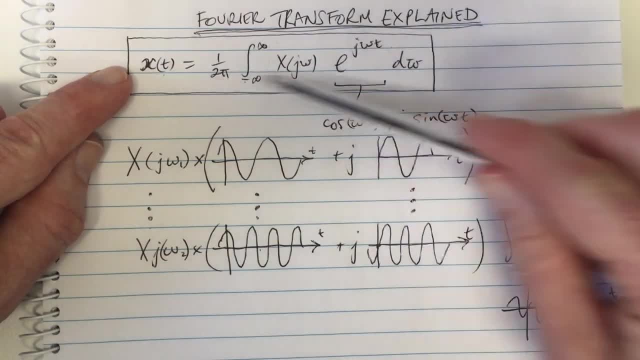 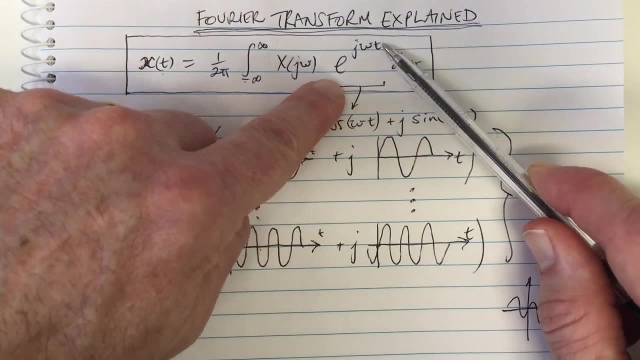 That's what this equation says. So, once again, to reiterate, when I see this equation, I really encourage you and I think about this as waveforms, These complex waveforms, all at their own value of omega. here they all are. 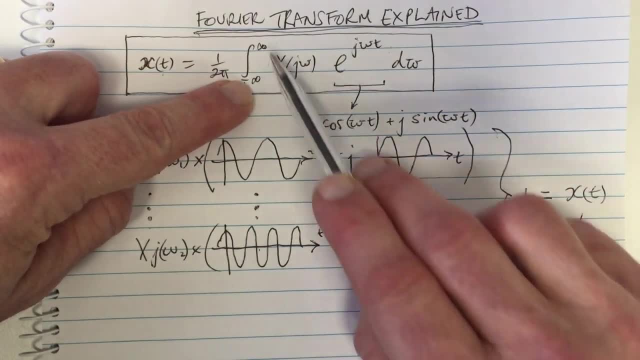 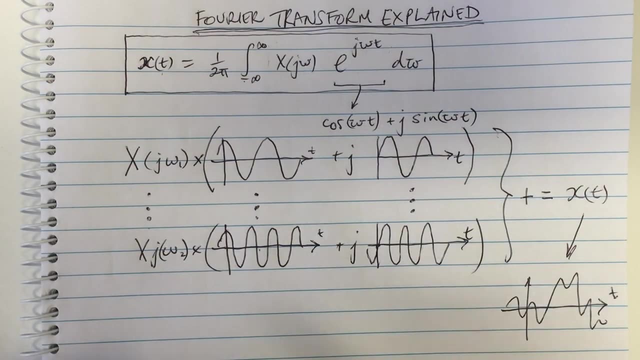 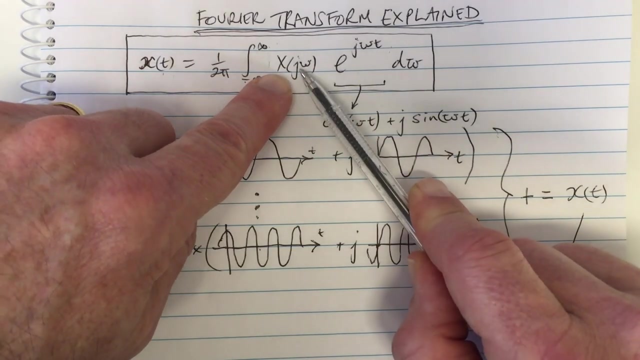 We're going to have them all at different values of omega. we're going to then add them all up from omega equals minus infinity to infinity, And this is the way to think of a Fourier transform. Our time domain signals are made up of amounts, of weighted amounts of each of these different 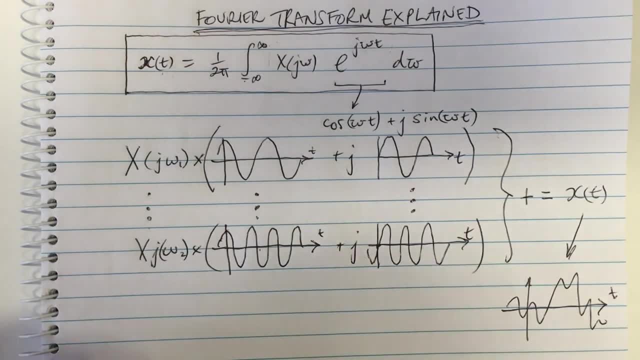 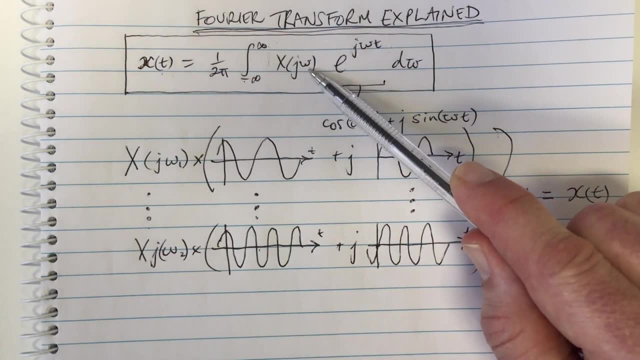 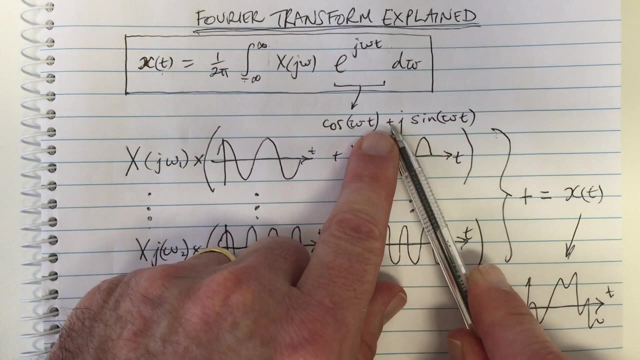 basis functions. And these are the basis functions. An interesting thing is, if you have a symmetric function here, if this is symmetric with negative frequency and positive frequency, then you'll have negative omegas, And the negative omega means that there's a minus out in front of the signs. 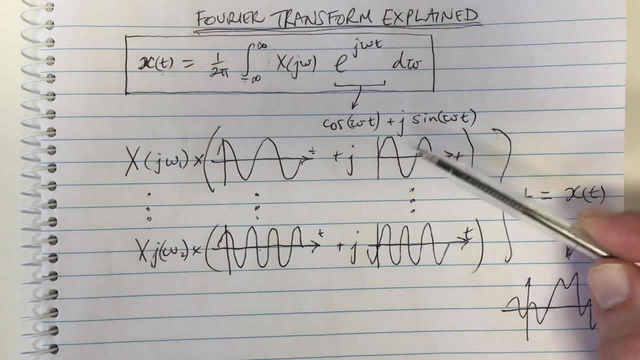 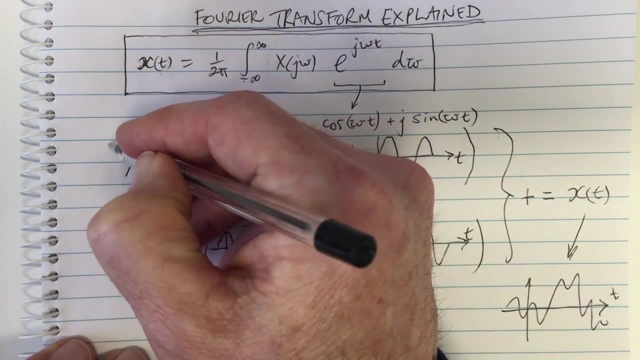 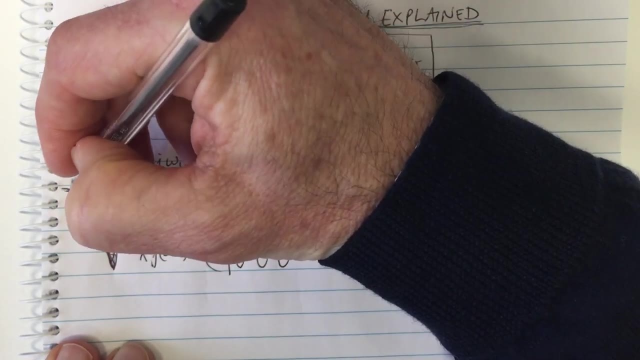 So it means that the negative in the sign will cancel the positive in the sign, And so you're only left with a real valued signal. Another thing to point out is if we go down in this direction here and if we plot it in this direction and we sort of turn this on the side and plot in this direction here,